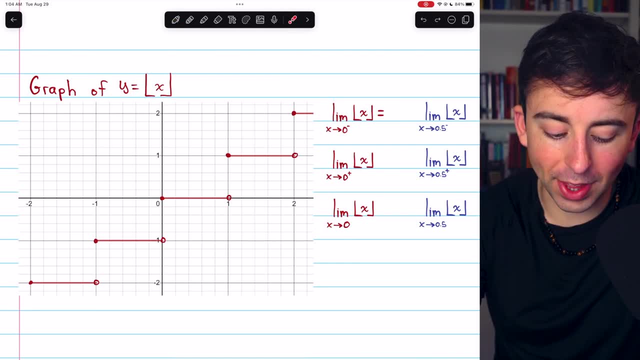 is what? Well, if we're approaching 0 from the left, we're over here And we can see that immediately to the left of 0, the function is equal to negative 1.. So this limit is negative 1.. On the other hand, if we approach 0 from the right, we can see: 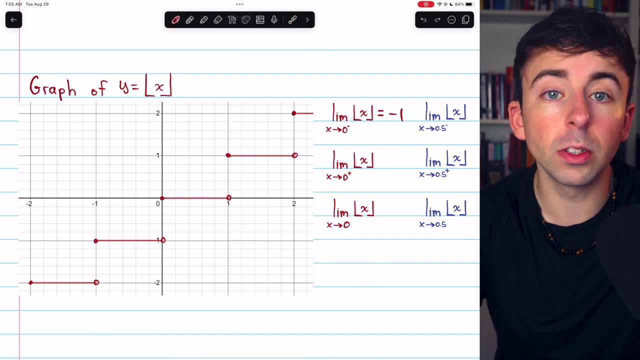 immediately to the right of 0, the function is equal to 0. All of those numbers that are a little bit bigger than 0 get rounded down to 0. So this limit is 0. This means the two-sided limit. 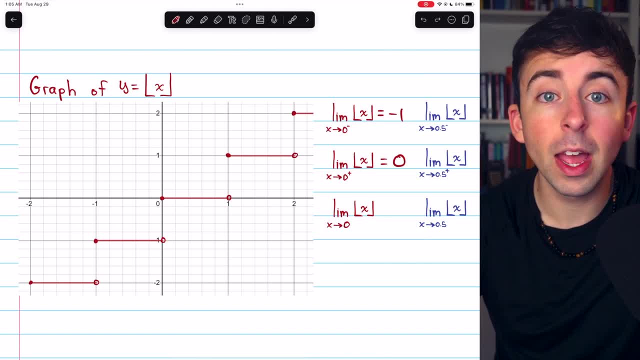 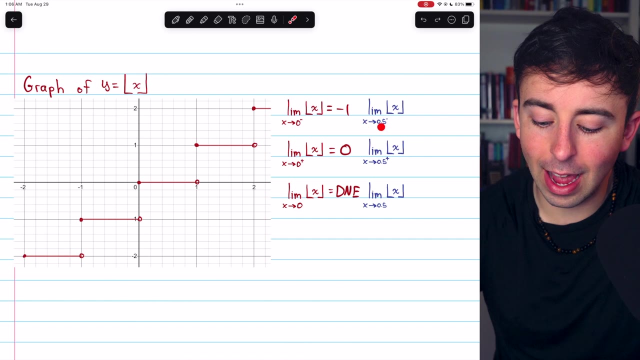 the limit of the floor function, or greatest integer function as x approaches 0, without regard to side, does not exist because the one-sided limits left and right are different. On the other hand, what about the limit of the greatest integer function as x approaches a? 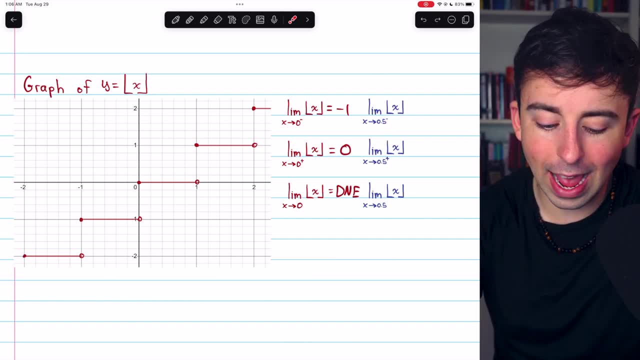 non-integer value. As x approaches 1 half, for example, from the left, 1 half is right about there. From the left, we can see that the function is equal to 0.. From the right, if we approach 1 half. 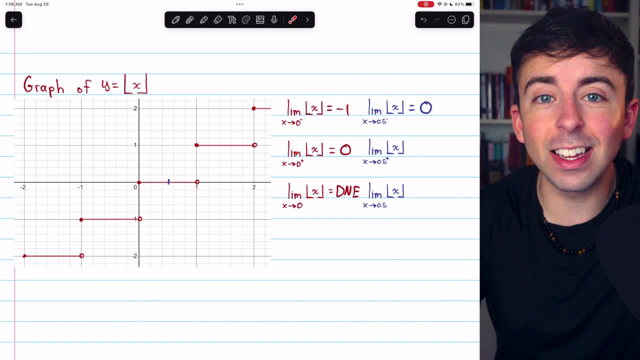 still, the function is equal to 0.. Anything near 1 half, whether it's to the left or to the right, is getting rounded down to 0.. And so this two-sided limit, the limit of the greatest integer function, as x approaches 1 half. 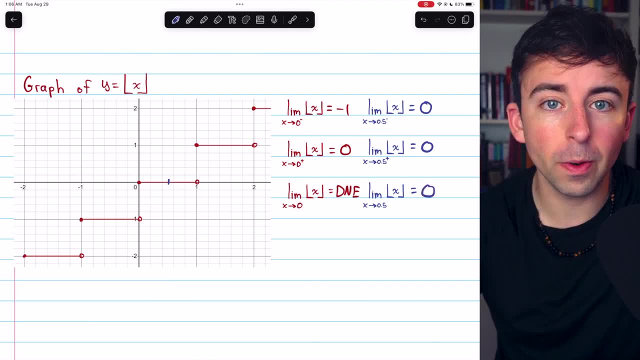 does exist and it's equal to 0.. A similar thing will happen with any limit of the greatest integer function as x approaches a non-integer value. If x was approaching 0.9,, for example, the limit would still be 0, because whether we're approaching 0 or 0,, the limit would still be 0,. 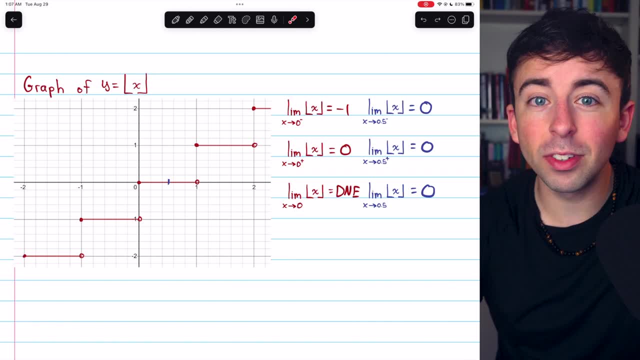 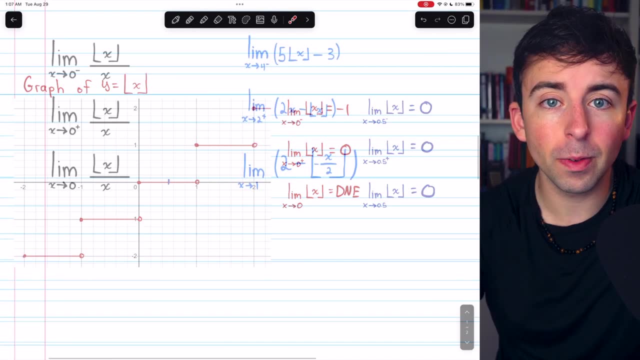 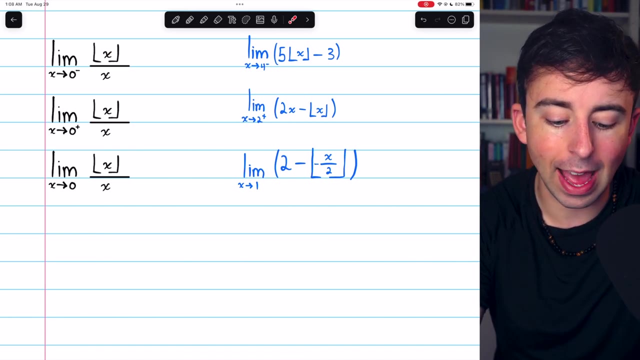 Portion of Y of the x-axis greater than or equal to 0.. From here, this experiment would be greater than or equal to the number of elements in the- Let's do this- handful of additional examples. We'll look at a graph of this function: the floor of x divided by x. after evaluating the limits. 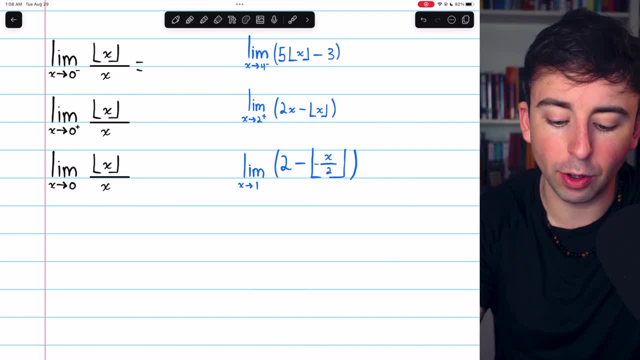 Let's just consider how to think through these, even if we don't have a graph. The limit of the floor of x divided by x, as x approaches 0.. The above exampleil lets us consider how to think through these, even if we don't have a graph. 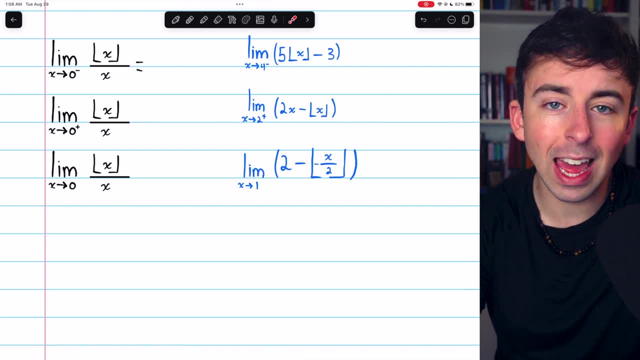 The limit of the floor of x divided by x as x approaches 1 half, x approaches 0 from the left. is what In the numerator, the greatest integer function of x as x approaches 0 from the left? we're going to be plugging in these really small. 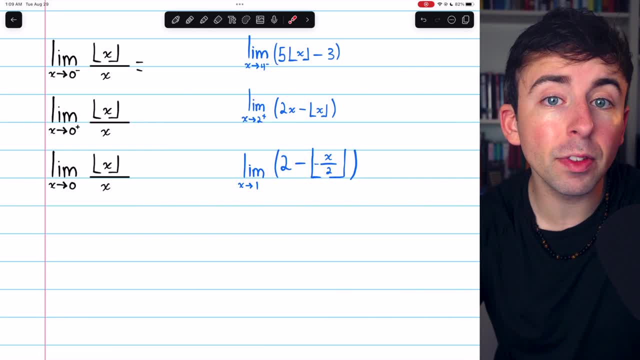 negative numbers. They're approaching 0, but they're to the left of 0. So they're small negative numbers which will all get rounded down to negative 1.. So this numerator would just equal negative 1.. The denominator is just x, so clearly it's approaching 0 from. 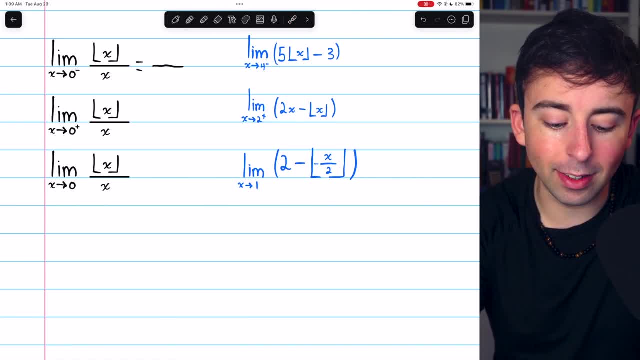 the left. Thus what we really have is negative 1 divided by really small negative numbers. The negatives will cancel out, and thus this limit will be going to positive infinity. We could also say: the limit does not exist, but this is exactly how it doesn't exist. 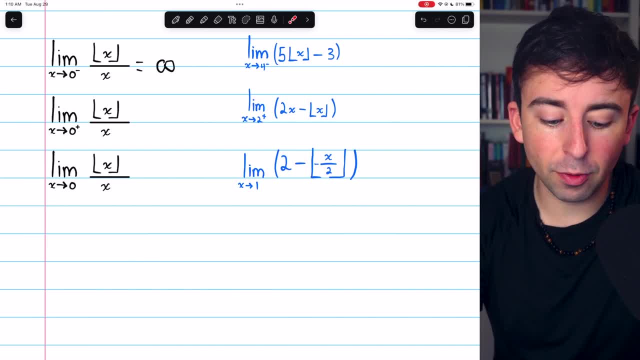 It's going off to positive infinity Again. that's because the numerator is a finite negative negative- 1, and the denominator is negatives that are getting closer and closer to 0. The negatives cancel out. We have a finite number divided by arbitrarily small numbers. It's going to infinity. 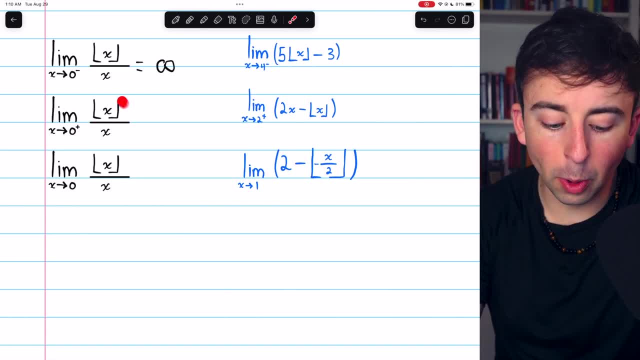 Now, if we approach 0 from the right in the numerator, we'll be plugging in very small positive numbers into the greatest integer function and those will all be rounded down to 0. The denominator will be approaching 0, but all of those numbers will be positive because 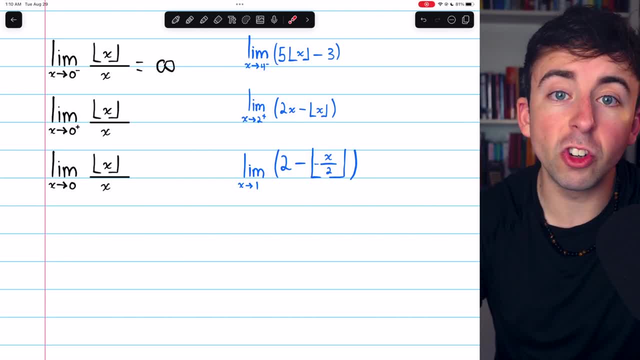 we're approaching 0 from the right. So we have the numerator, which equals 0, exactly divided by numbers that are approaching 0 and are positive. Thus this limit equals 0.. Thus the two-sided limit we can say does not exist, because from the left the function's 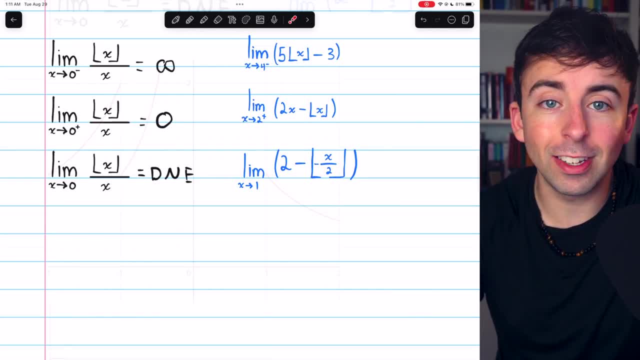 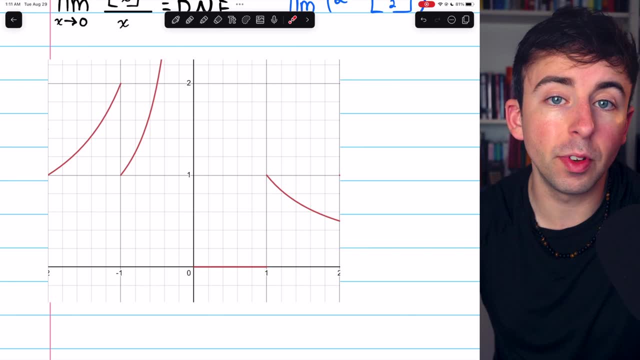 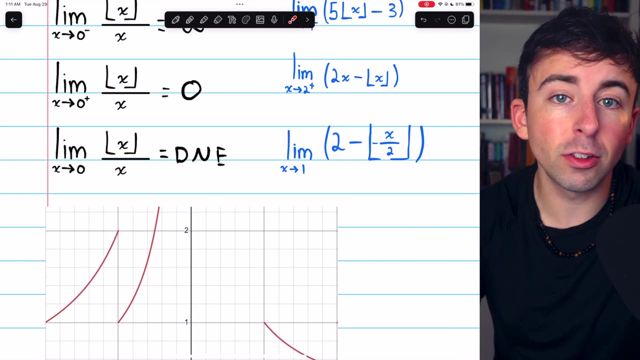 approaching positive infinity and from the right, it's approaching 0.. And here is a graph where we can see that, As we approach 0, from the left the function is going off to positive infinity And from the right, like we said, it's equal to 0, because these numerators are just small: positive. 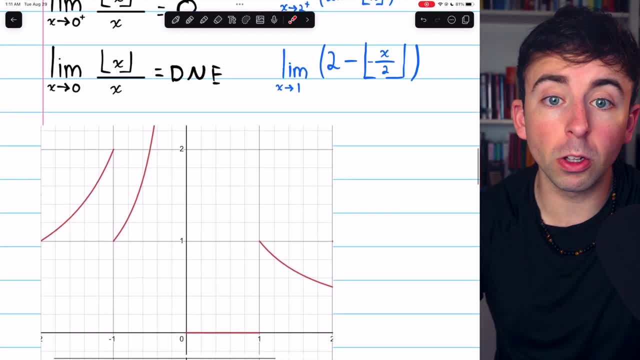 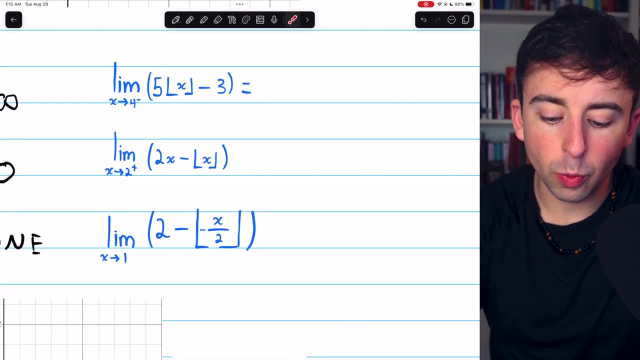 numbers getting plugged into the greatest integer function. Those are all going to be rounded down exactly to 0. So we just have that flat line, All right, three more basic examples here. We just have to think carefully about how the greatest integer function works. 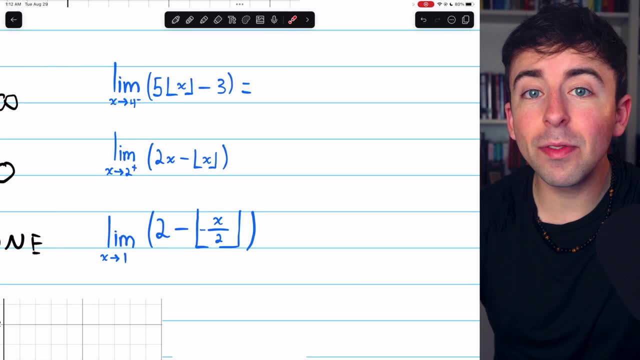 Here x is approaching 4 from the left, So we have numbers that are close to 4, but there are less than 4,, which means the greatest integer function will be rounding all of those down to 3.. Thus, this is just going to be. 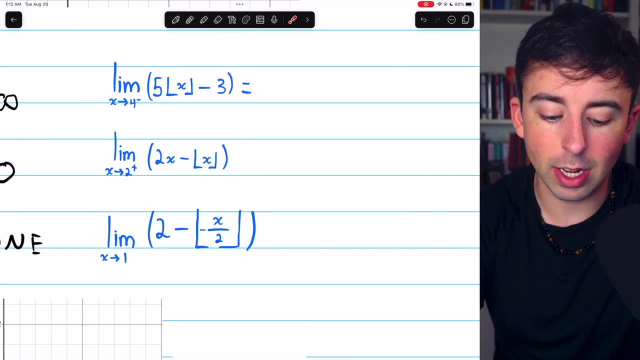 5 times 3, which is 15 minus 3,, giving us 12.. In the next problem, x is approaching 2 from the right. So when we plug that in to the greatest integer function, we're plugging numbers in that are a little bigger than 2.. 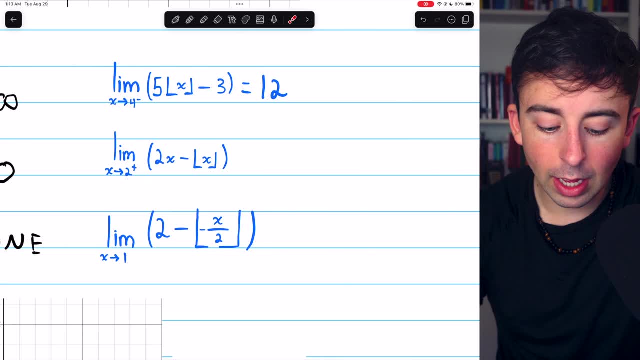 Thus, we're going to be rounding all of those down to 3.. And we're going to be rounding down to 2.. So we have 2 times x, which is essentially 2 times 2, because x is approaching 2.. 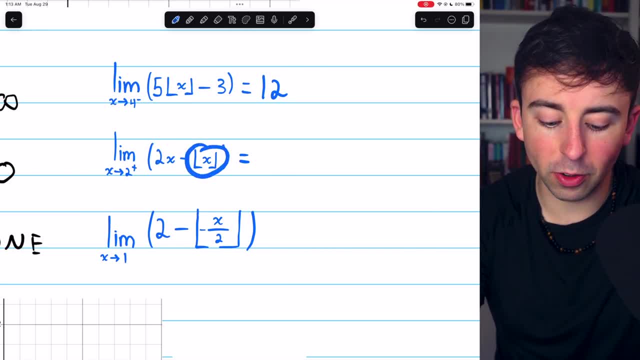 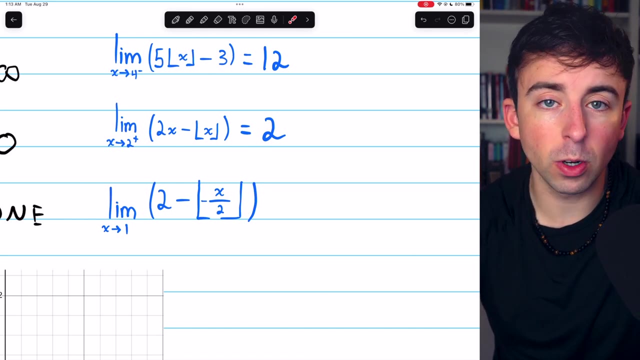 So that's 4.. But then the greatest integer function, that's going to round down to 2 every time. So this is just equal to 4 minus 2, which is 2.. Finally, the limit of 2 minus the floor of negative x over 2, as x approaches 1.. 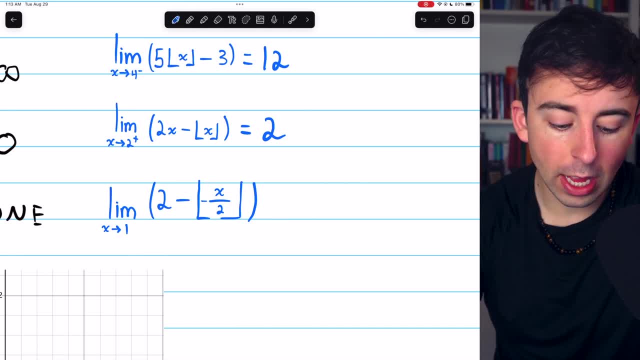 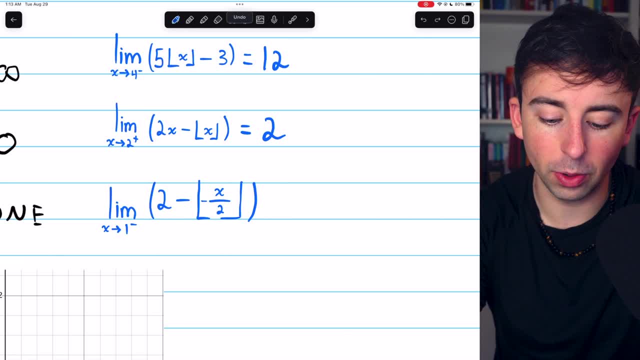 Let's begin with x approaching 1 from the left, so I'll denote that here We're looking as x approaches 1 from the left. Since x is approaching 1 from the left, these x values will be close to 1.. 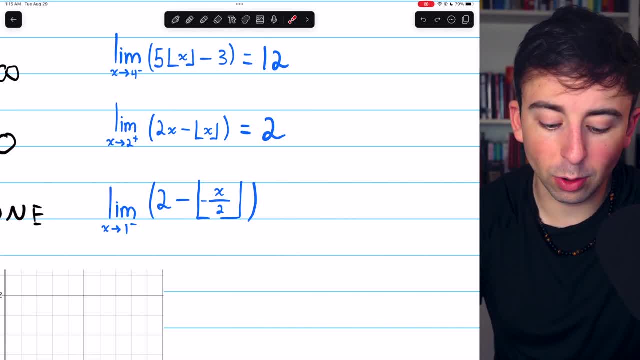 However, they will be less than 1.. So this x over 2 will be approaching 1 half, But then it's getting multiplied by a negative, so it's approaching negative 1 half, But then the floor function will round negative 1 half down to negative 1,. 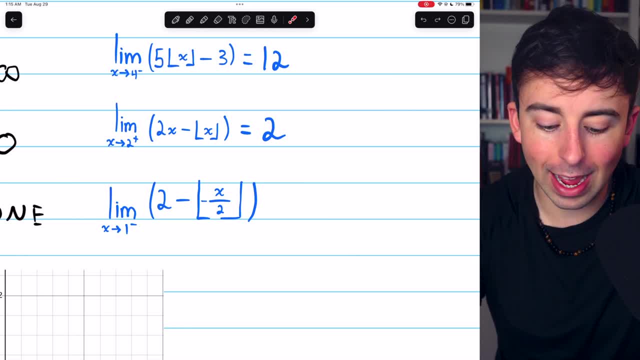 the greatest integer less than or equal to negative 1 half. So this is 2 minus negative 1, which is going to be 2 plus 1,, which is 3.. That's the left-hand limit. Now, if x is approaching 1 from the right, 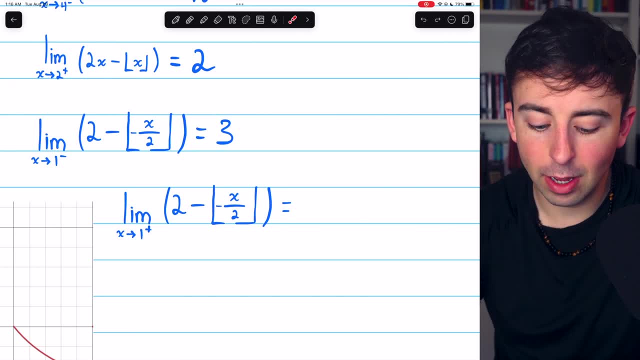 well, x over 2 will still be 1 half, but then we multiply it by a negative, so it's negative 1 half. The greatest integer function rounds that down to negative 1, and again it's approaching positive 3..